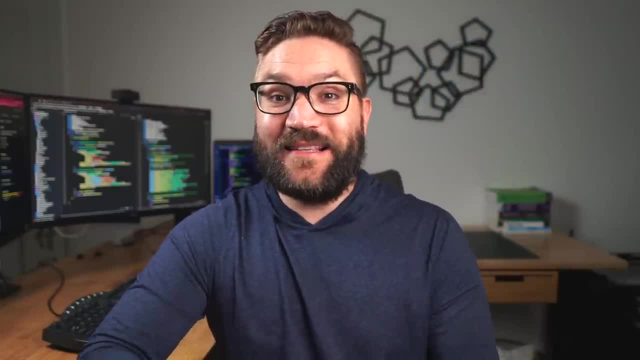 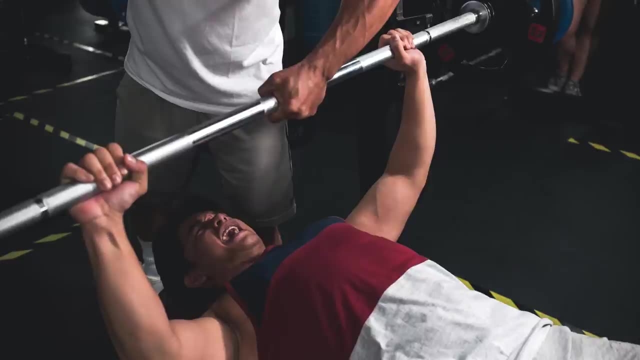 recommending C++ as your first programming language because they'll say something like this is the right way to learn programming. To me, that thinking is like if you hire a personal trainer to get in shape and tell them the only way you can get in shape is if you start bench. 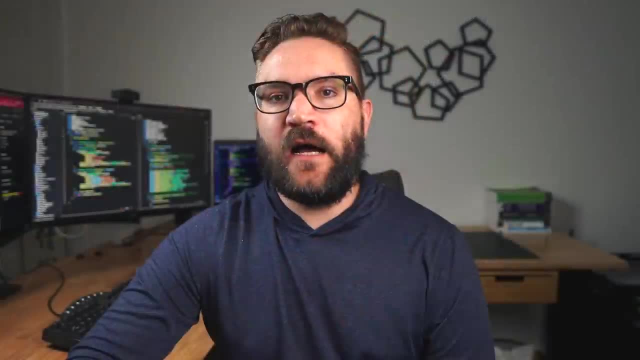 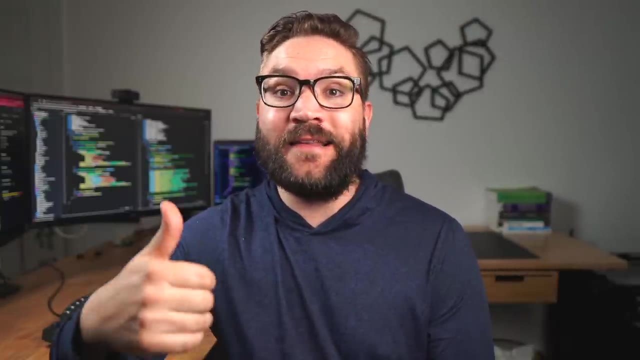 pressing 500 pounds right away. It's just too much. C++ is not your average programming language. It's a low-level programming language, which means that it has direct access to a computer's resources, such as memory and CPU registers. This means that you, as a programmer, have to learn how. 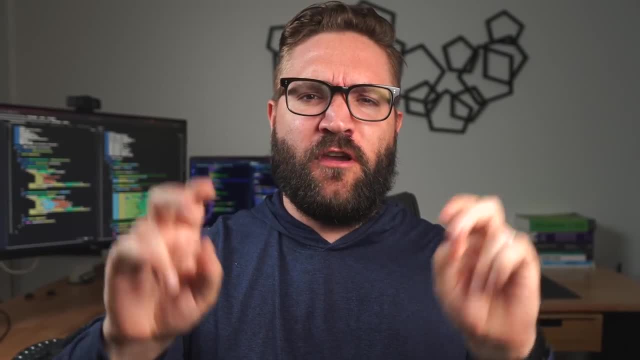 memory management works and other things like that. So if you're a programmer and you're a low-level tasks, this is a good thing, many seasoned programmers will say. But in reality, for many of you, just learning the fundamentals of how programming works is hard enough. We don't. 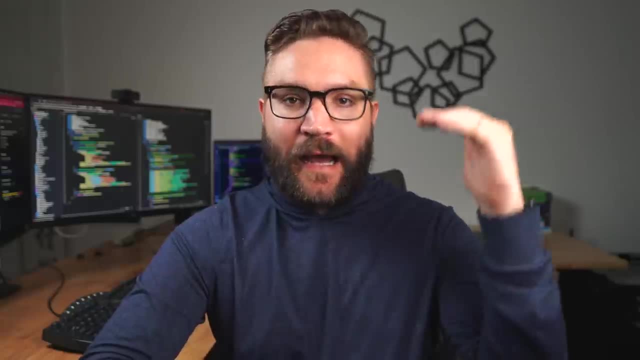 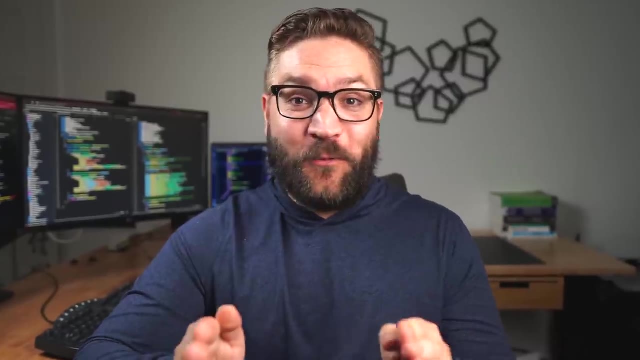 have to add anything else more advanced on there. It's better instead to pick a high-level programming language like Python, where you don't have direct access to resources and you don't have to learn about memory management. Now, that being said, if you personally have an indomitable will, 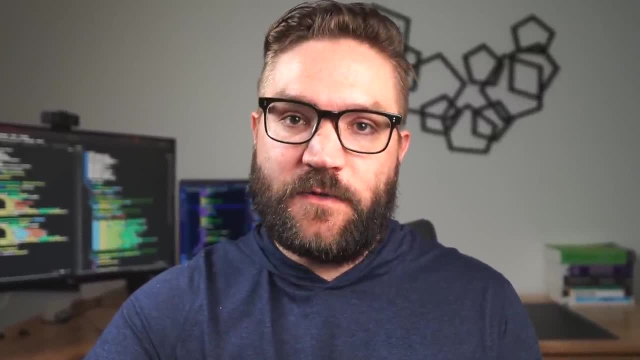 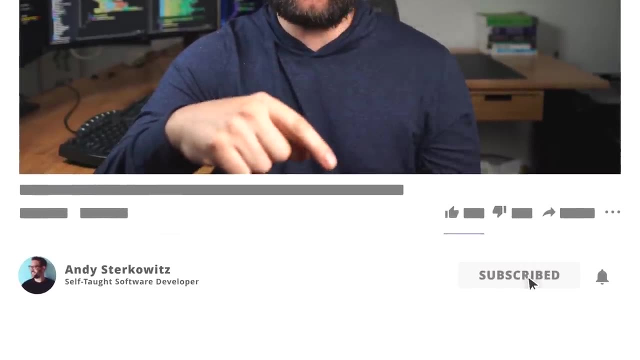 you have patience and you have a lot of time in your hands, then go ahead and choose C++. Now, have I insulted you yet by tearing down your favorite programming language? If the answer is no, then what you should probably do is go down and hit that subscribe button, because I want to get. 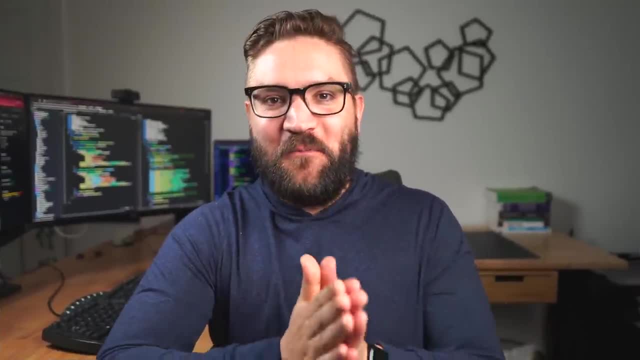 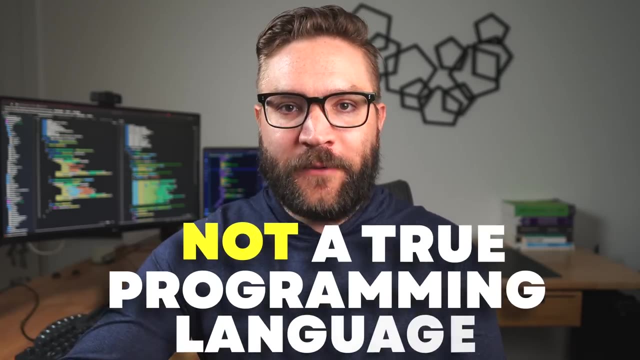 your subscription before I completely alienate you. So, moving on here, Another language you'll often hear recommended is SQL, pronounced sequel. You should not learn this first, because, well, for one, it's not a true programming language, It's actually a query language. A query language. 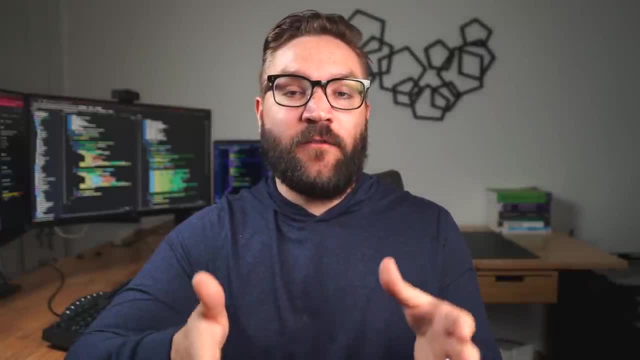 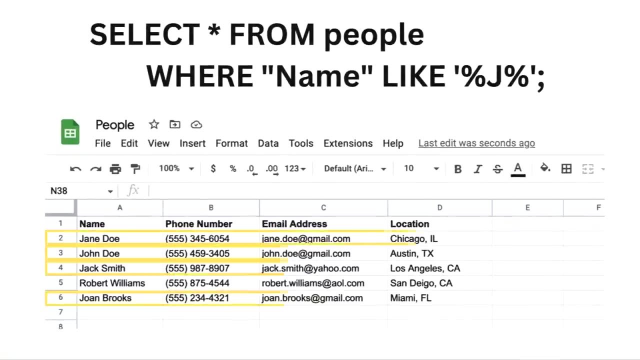 has some programmatic aspects, but its main purpose is to query data from relational databases. And for those of you who are non-techie, a database is kind of like an Excel spreadsheet in that query language is really good at filtering out information, inserting information, et cetera, et cetera. Now 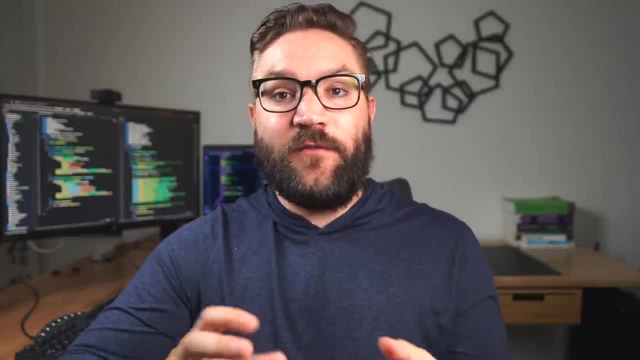 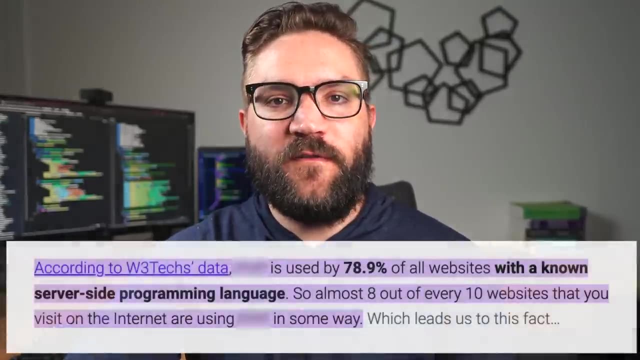 down the line, learning SQL once you have some programming experience and you have a need for a database, but for now skip it. The next programming language I'm actually going to recommend avoiding is a very widely used programming language, According to some of 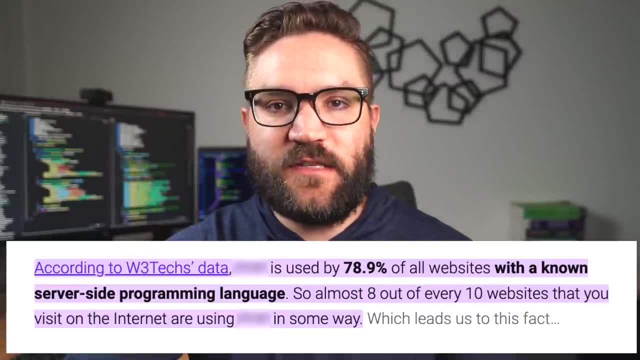 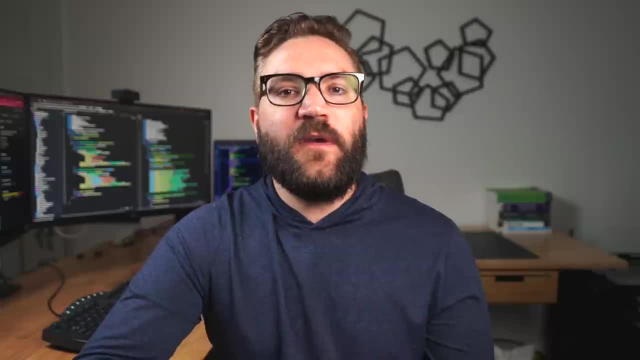 the statistics I've seen, this programming language is used in something like 70% plus of websites that you visit. The language, of course, that I'm talking about is PHP. Now why on earth would you want to avoid something that's so widely used? For two main reasons. 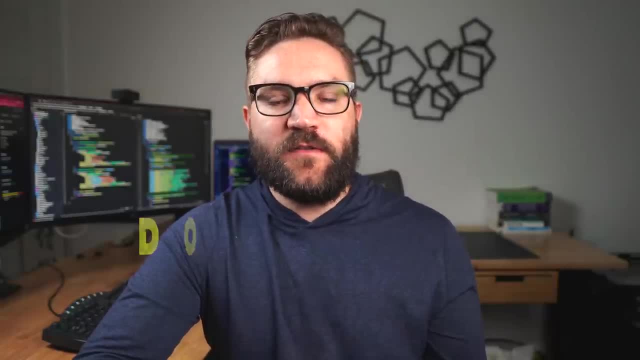 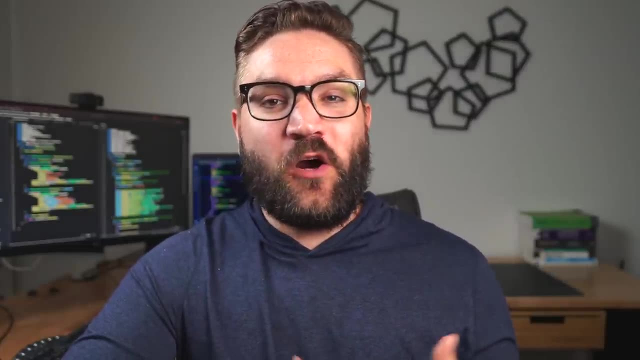 Number one: the first language that you learn may not be the one that you land a job with, So you don't want to choose a programming language solely on popularity. And number two is it suffers from problems of C-sharp and Java, meaning it's hard to get set up, Like I remember way back when 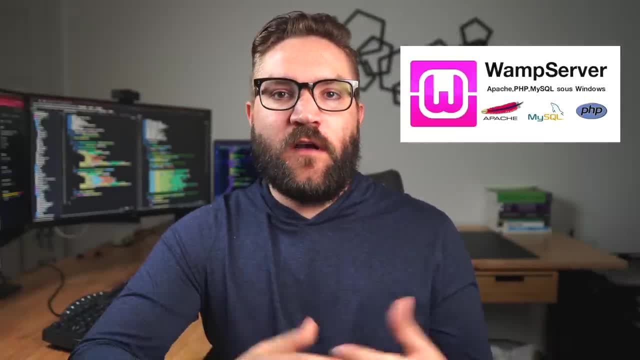 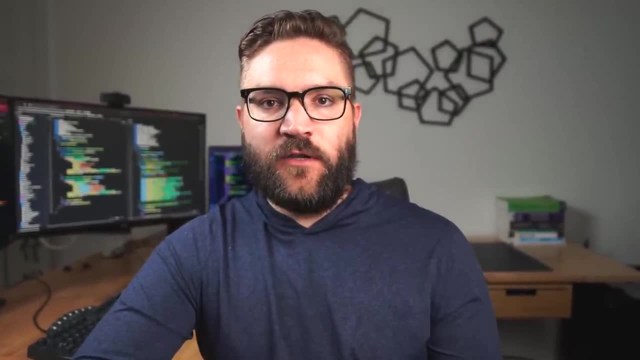 when I was first learning, it was very hard for me to set up a Womp server And it's also difficult to start getting projects under running with PHP. With all that being said, I think PHP is an excellent second language to learn, Despite what you may hear online. a lot of professional 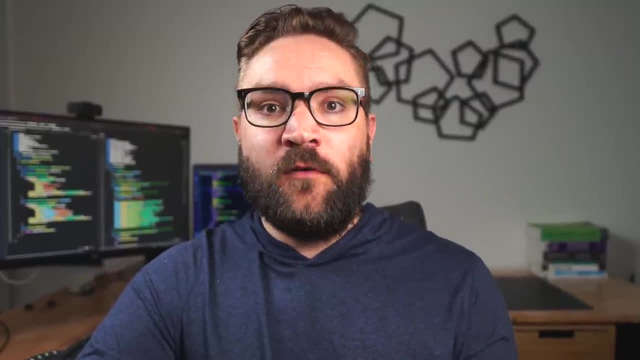 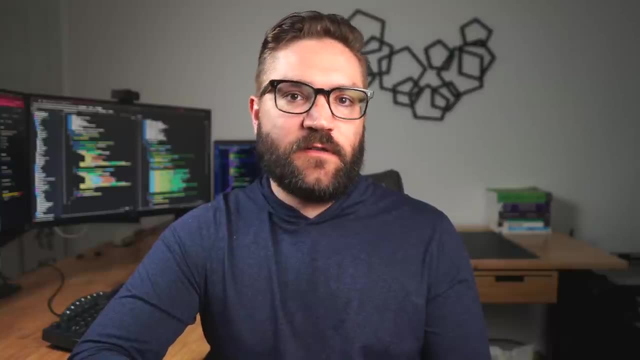 developers hate it. What I have found is that the syntax is actually quite readable for new developers, and using something like the layerable framework is pretty helpful for developing a nifty web app. So choose something else first. learn PHP later on. All right, So I'm going to continue. many of you here and say that the next two languages that you should avoid are Swift and Kotlin. Both of these languages are primarily used for mobile app development, with Swift being for iOS and Mac OS and Kotlin being for Android. The thing is, I found that both of these programming 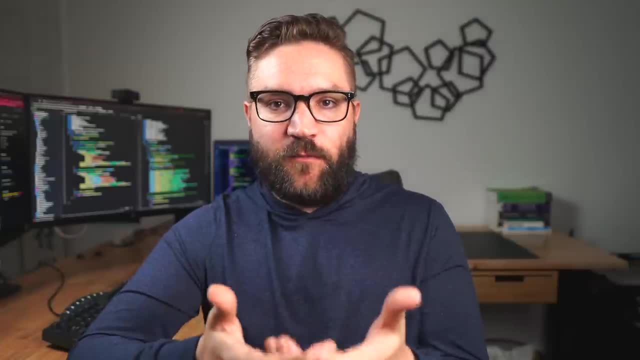 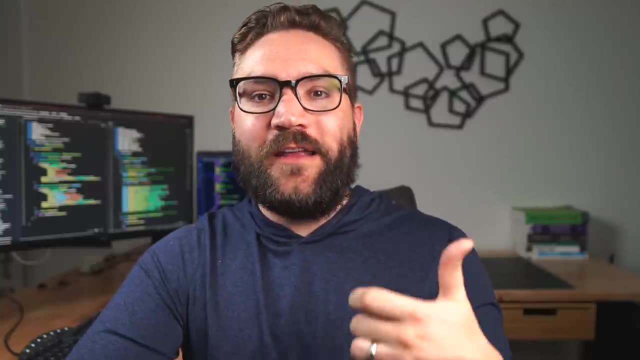 languages are excellent to learn once you have a foundational skill set with programming, but it suffers from the same problems as many of the other programming languages I've talked about, The main one being that it's hard to get up and running. You have to get handheld through so many 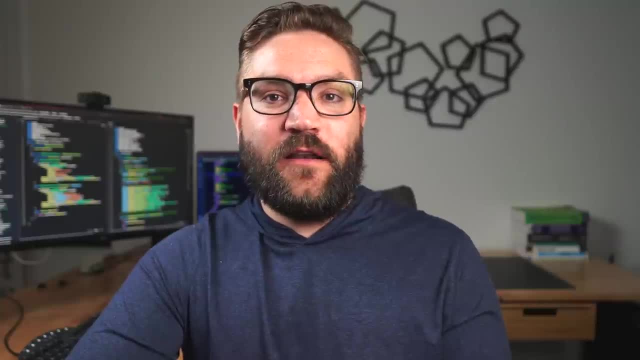 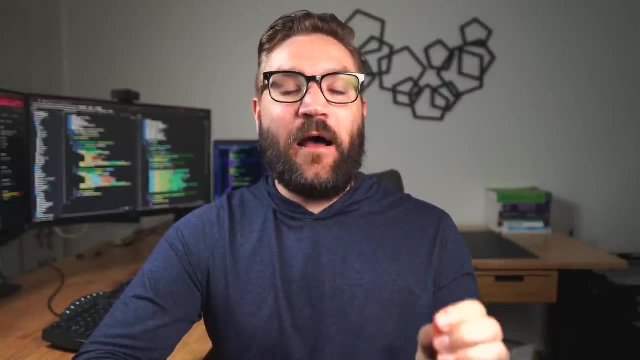 tutorials And even coming up with project ideas to get started is a hard and difficult process. The only people I think would benefit from Swift or Kotlin as a first programming language is somebody who is dead set on being a native mobile developer, So somebody has no interest in web development or 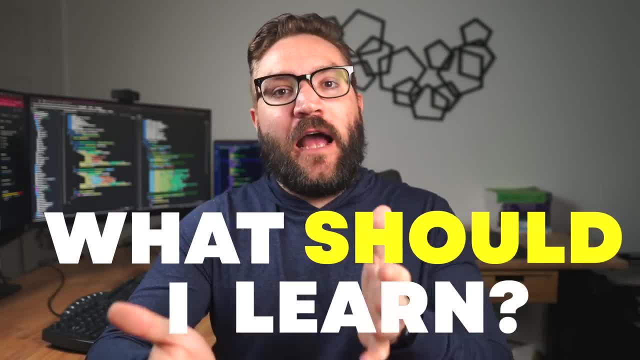 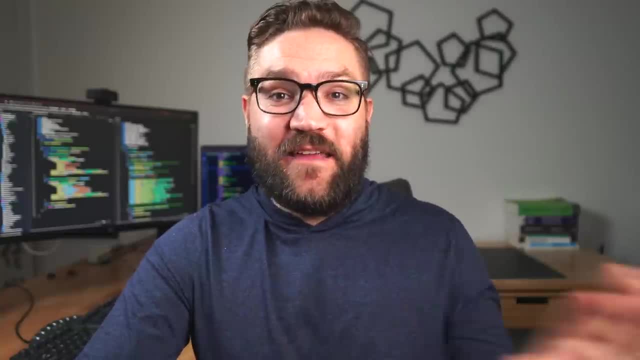 anything like that. That leaves us with one last question, which is: what should I learn? I've alluded to it before, but I think Python and JavaScript are both excellent languages. I personally recommend JavaScript, But keep in mind, you could pick any of the programming languages. 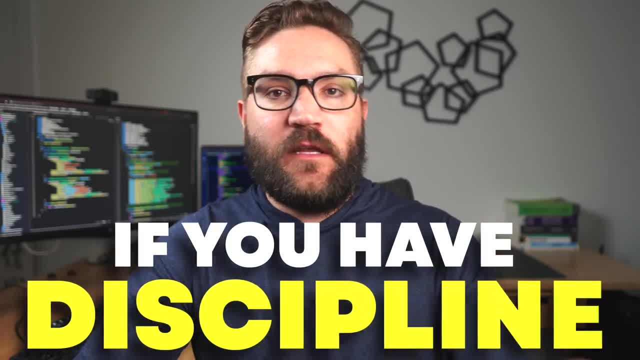 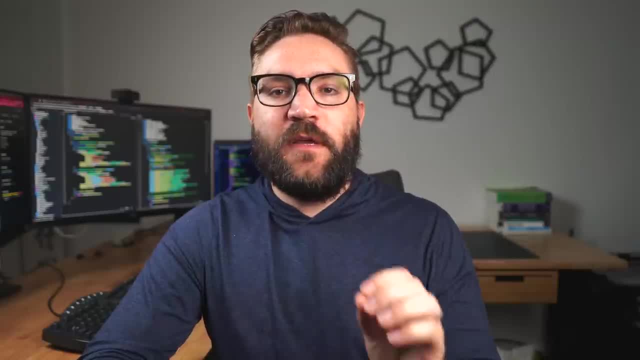 that I said not to learn, and you can still be successful. If you have discipline, if you have grit, if you can commit to this for a long period of time, you can be successful with anything. The first programming language shouldn't be complicated, so don't overthink this Pick. 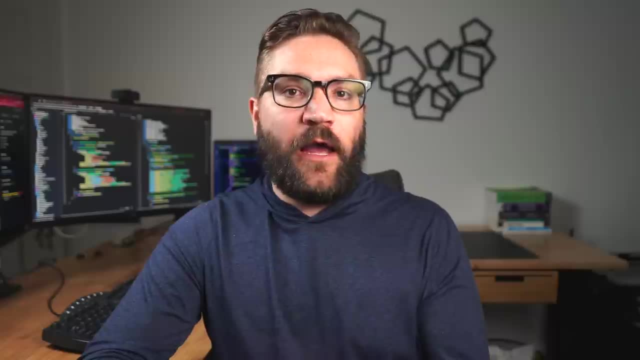 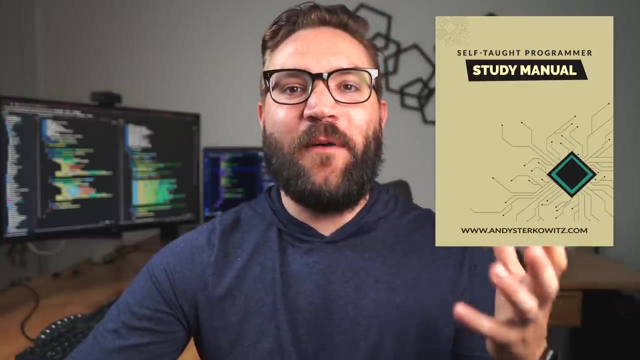 something. stick to it for two or three months. learn as much as you can. I promise you good things will happen. By the way, you should know I've created a free PDF called the Self-taught Programmer Study Manual. I've tried to put as much wisdom as I could about how to be a self-taught. 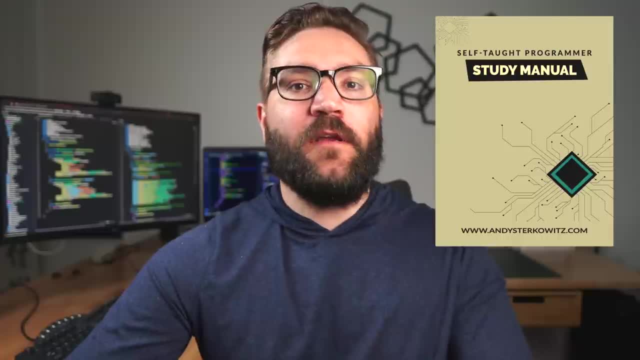 programmer how to get the most out of your studying. If you want a copy of that free PDF, I will leave a link in the description below of how you can access that. Other than that, thank you so much for watching Peace out everybody. 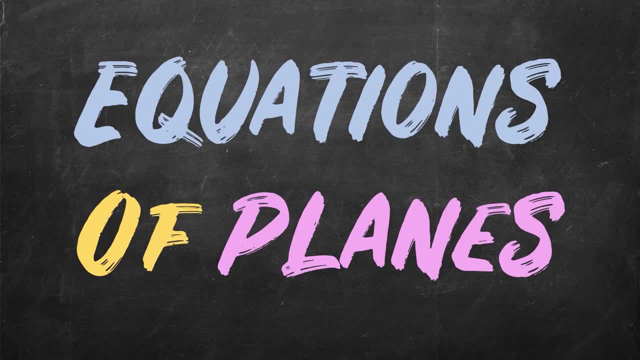 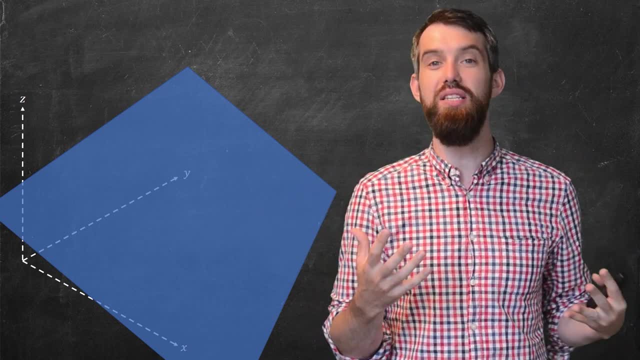 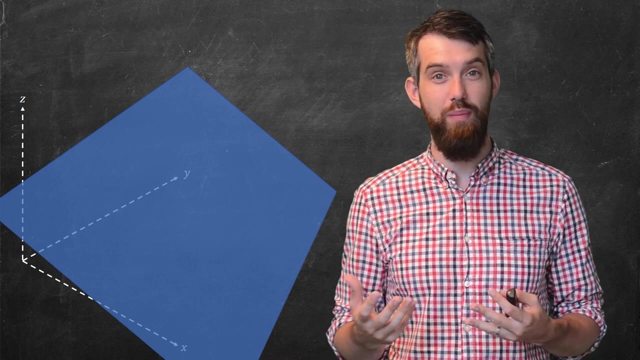 In this video we're going to come up with equations for planes like this, and it's going to sort of extend the work that we did previously on equations for lines. Now, when we did equations of lines, I had to give you a couple pieces of information.